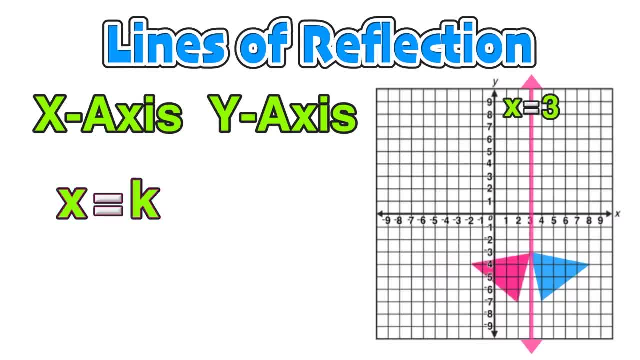 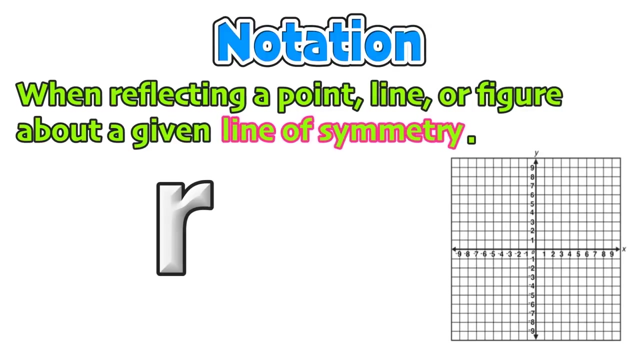 The vertical line equation X equals K. in this case, K equals 3.. The horizontal line equation Y equals K. in this case, Y equals negative. 2. The line Y equals X And the line y equals negative x. When reflecting a point, line or figure about a given line of symmetry, we use the lower. 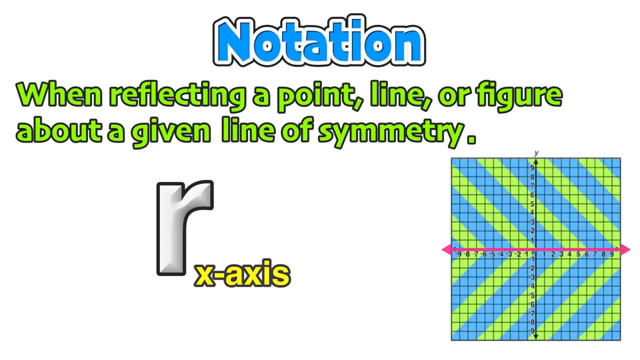 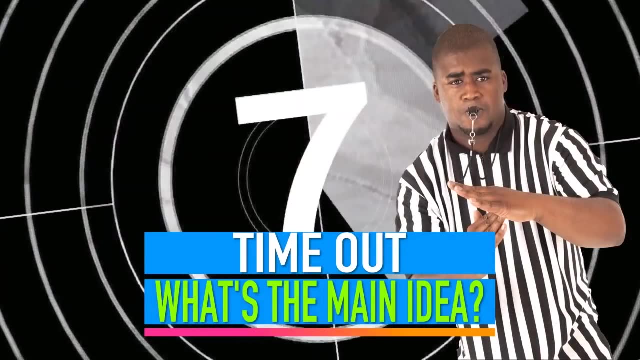 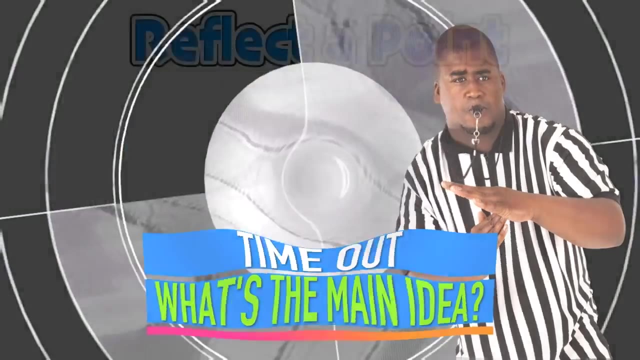 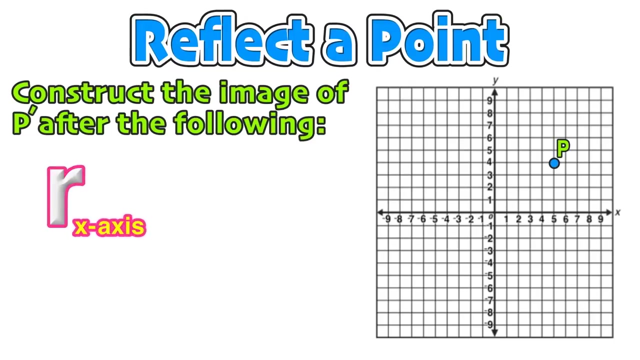 case r notation. This notation will specify the line of symmetry for which our reflection will occur. For our first example, we will be reflecting a point. Notice that our line of symmetry is the x-axis. This is the line that we are going to be reflecting our point P, with coordinates across. 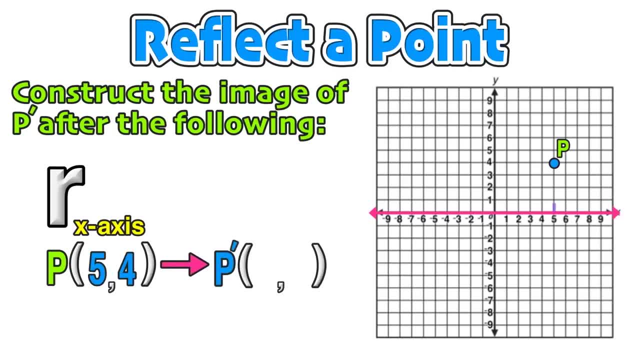 To find the coordinates of the image P' we will count how many units the point P is away from the line of symmetry, in this case 4 units. Next, we will count the same number of units on the other side of the line of symmetry. 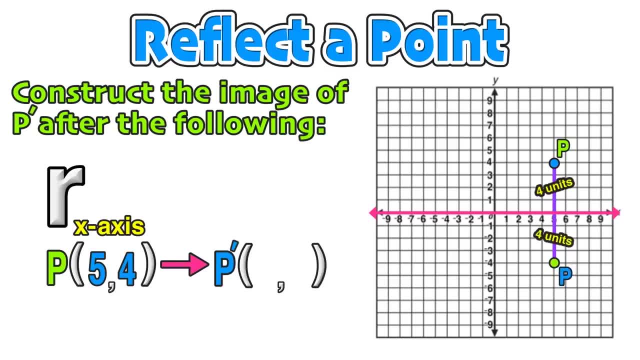 So again, 4 units. Now we have the location of the point P' with coordinates. When reflecting over the x-axis, we should notice that the value of the x-coordinate did not change. however, the value of the y-coordinate was negated, going from 4 to negative 4.. 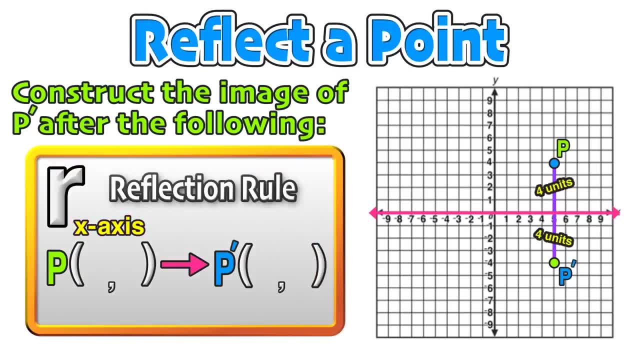 This reflection rule applies to reflecting any point over the x-axis and where the coordinates xy will become x negative y, Meaning that the value of the y-coordinate is negated. Now we can take a look at the next example. Let's look at the next example. 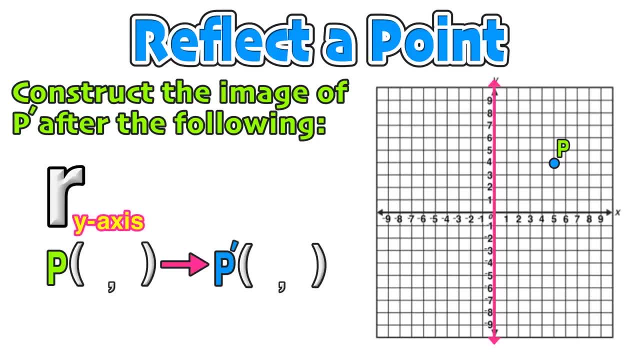 Let's take a look at taking that same point P and this time reflecting it over the y-axis. Our approach here is still the same: we are going to count how far away the point is from the line of symmetry, in this case 5 units. 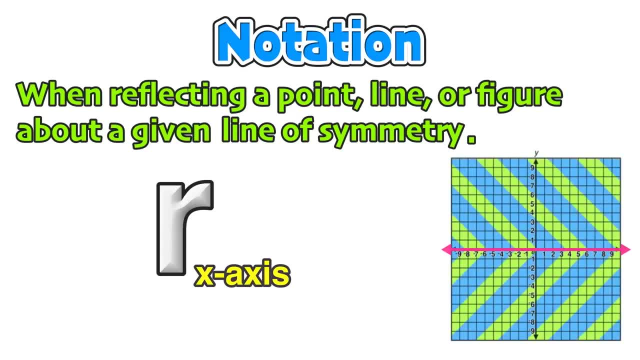 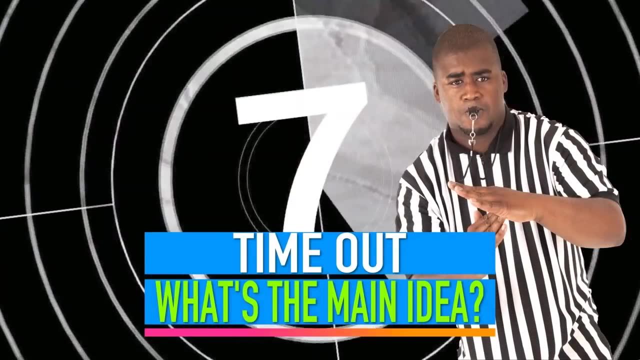 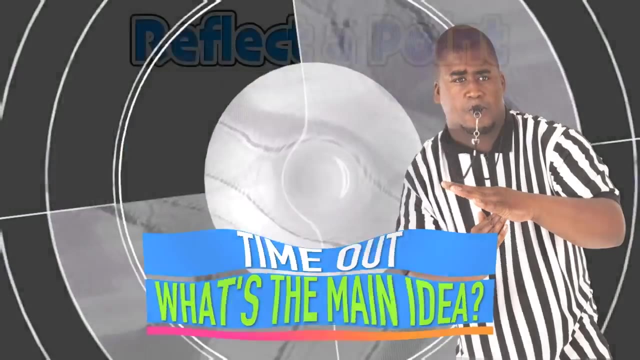 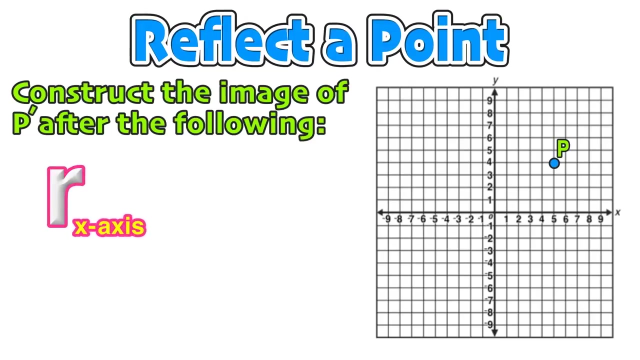 case r notation. This notation will specify the line of symmetry for which our reflection will occur. Haha, cool. For our first example, we will be reflecting a point. Notice that our line of symmetry is the x-axis. this is the line that we are going to be reflecting. 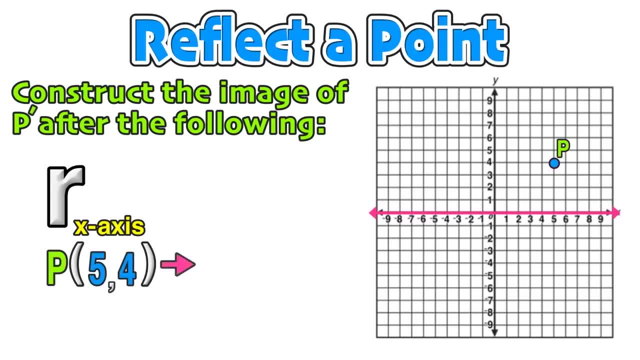 our point P with coordinates across. To find the coordinates of the image P' We will count how many units the point P is away from the line of symmetry, in this case four units. Next we will count the same number of units on the other side of the line of symmetry. 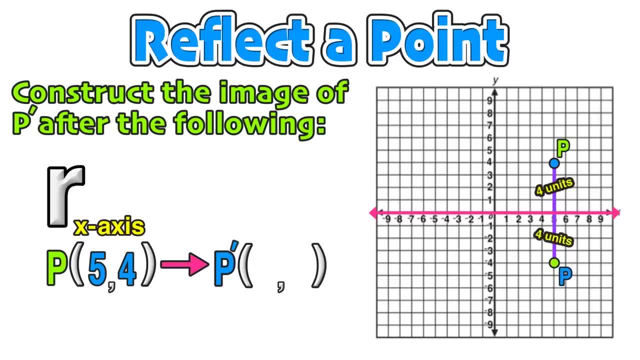 so again four units. Now we have the location of the point P' with coordinates five negative four. When reflecting over the x-axis, we should notice that the value of the x-coordinate did not change. However, the value of the x-coordinate did not change. 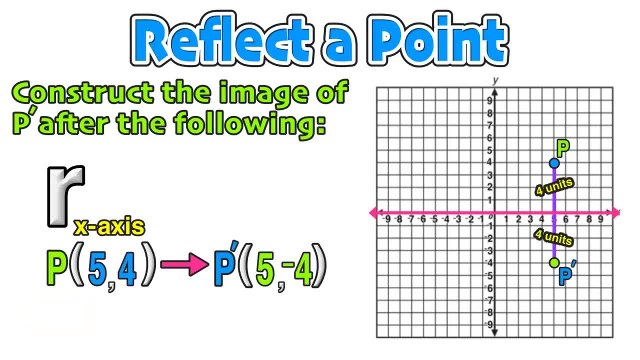 The value of the y-coordinate was negated, going from four to negative four. This reflection rule applies to reflecting any point over the x-axis where the coordinates xy will become x negative y, meaning that the value of the y-coordinate is negated. 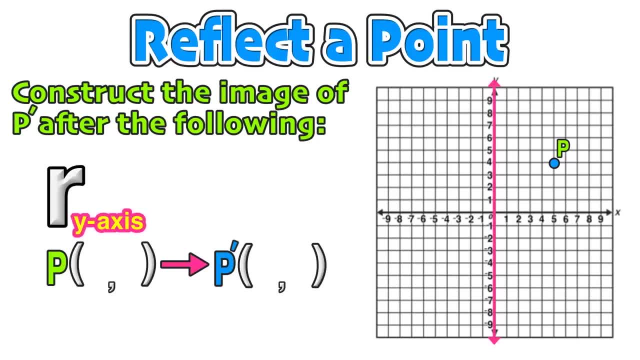 Now we can take a look at taking that same point P and this time reflecting it over the y-axis. Our approach here is still the same: We are going to count how far away the point is from the line of symmetry, in this case five units. 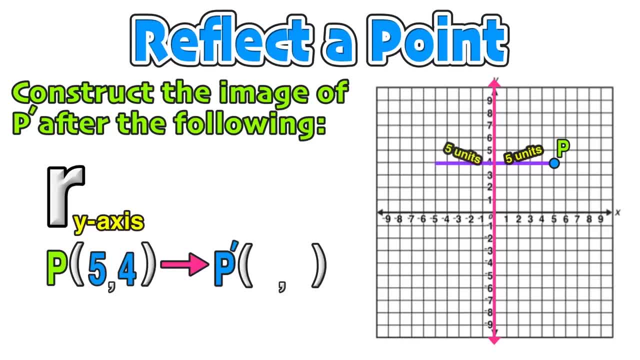 Then we can count the same amount of units on the other side of the line of reflection and plot the point P' The coordinates of this image at negative, five, positive, four. Notice that when reflecting over the y-axis, the x-coordinate value is negated and the 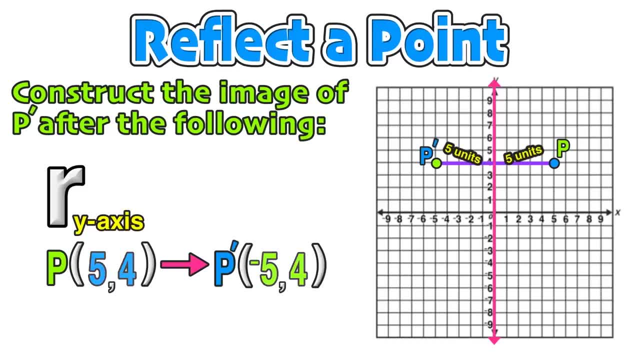 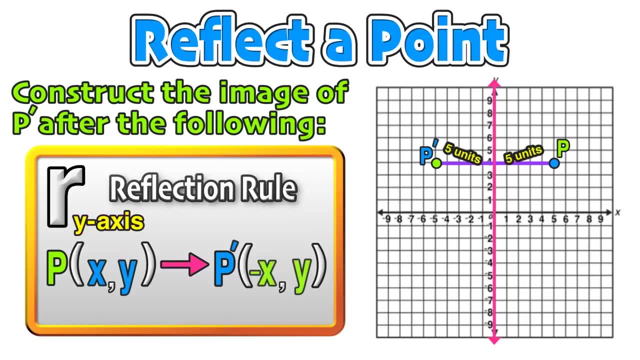 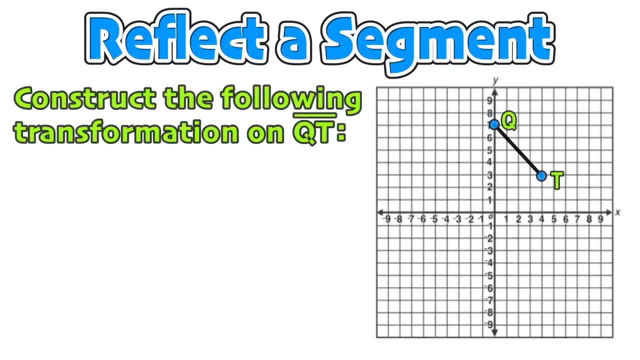 y-coordinate value is unchanged. In terms of a reflection rule, you can say that any point reflected over the y-axis with coordinates xy becomes negative xy where the x value is negated. For our next example, we are going to reflect a line segment. 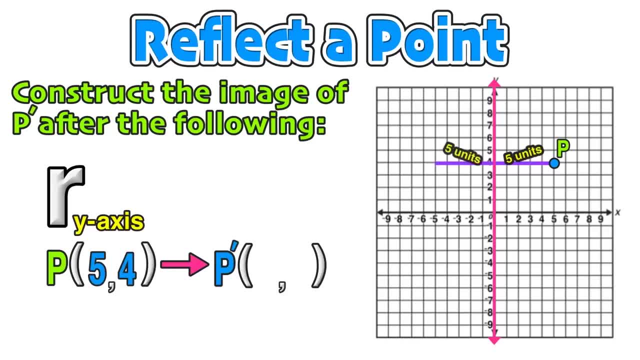 Then we can count the same amount of units on the other side of the line of reflection and plot the point P' The coordinates of this image at negative 5, positive 4.. Notice that when reflecting over the y-axis, the x-coordinate value is negated and the y-coordinate 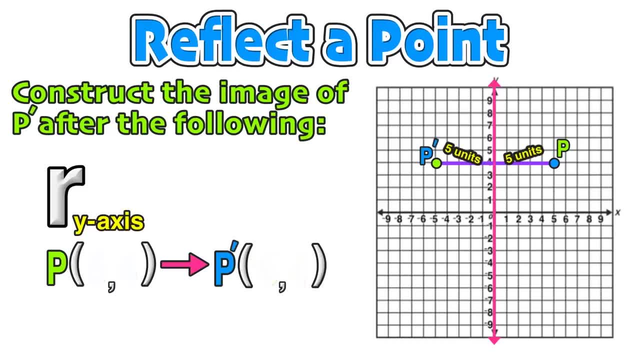 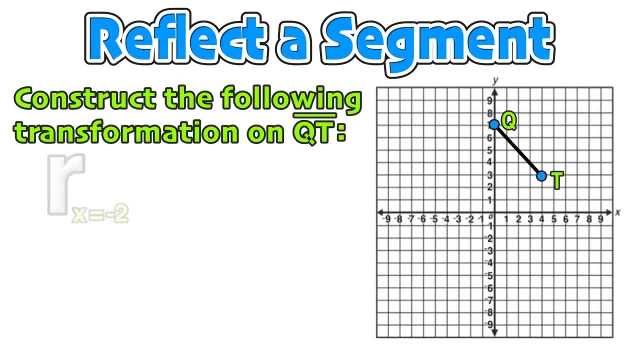 value is unchanged. In terms of a reflection rule, you can say that any point reflected over the y-axis with coordinates xy becomes negative xy where the x-value is negated. For our next example, we are going to reflect a line segment. 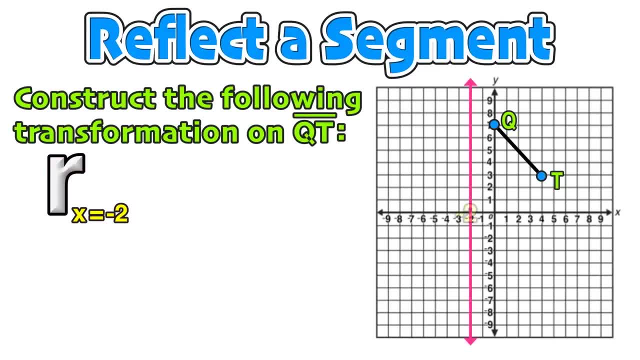 Our line of symmetry x equals negative 5.. The line of symmetry x equals negative 2 is a vertical line equation. Let's start by writing down the coordinates of the endpoints qt. To find the coordinates of the image q' we'll use the same strategy as the last. 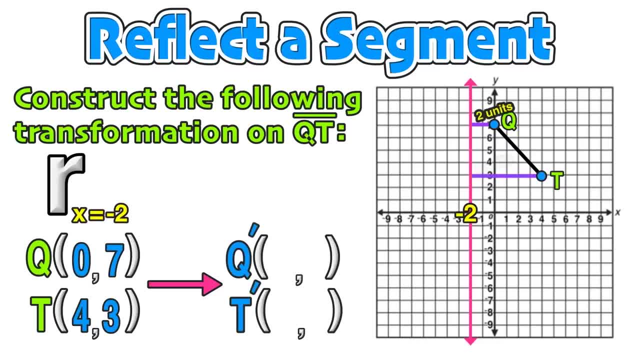 example, by counting how many units each endpoint is from the line of symmetry, We see that the point q is 2 units away from the line of symmetry. x equals negative 2, and the point t is 6 units away. The point t is 2 units away from the line of symmetry, x equals negative 2, and the point t is 6 units away. 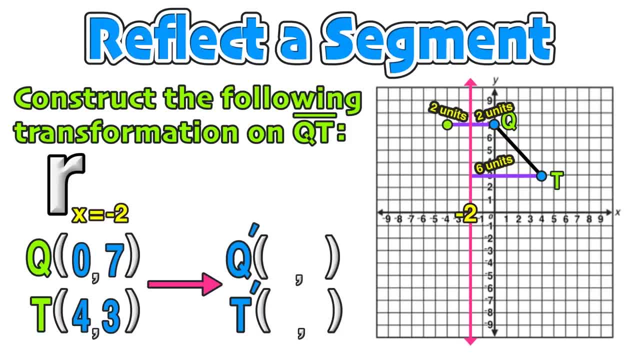 We can go ahead and repeat those distances on the other side of the line of symmetry and plot the new points of q' and t'. Now we can construct the image of the reflected line segment q' has coordinates of negative 4,7 and t' has coordinates of negative 8,3.. 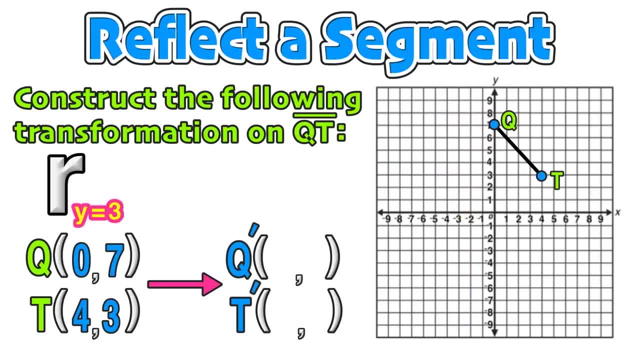 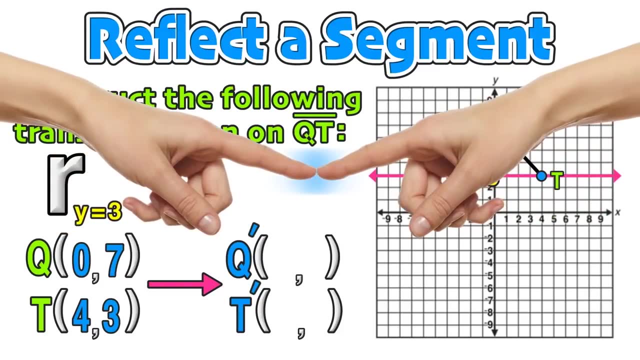 Now we can go ahead and try to reflect line segment qt over the line of symmetry yy. Notice here that the point t is directly on the line of symmetry, Just like pressing your finger up to the surface of a mirror and having it appear that another 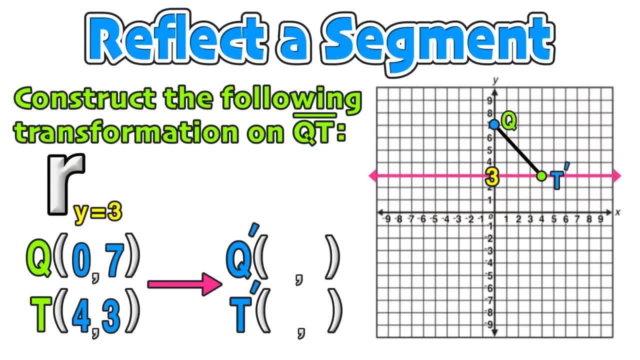 hand is directly touching it. having a point directly on the line of symmetry will have it stay on the line of symmetry, So t' will have the same coordinates as t. at Now the other end, point q, still needs to be reflected Again. we're just going to count how many units q is from the line of symmetry. 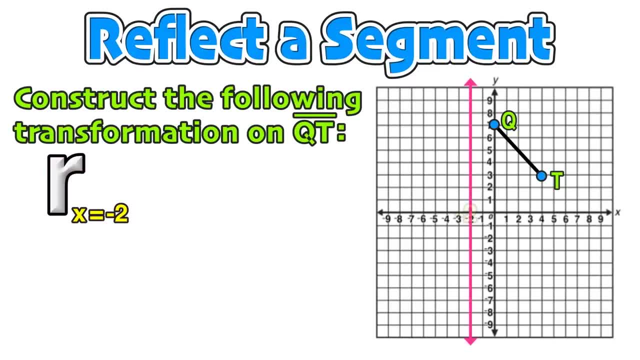 Our line of symmetry x equals negative. two is a vertical line equation. Let's start by writing down the coordinates of the endpoints qt To find the coordinates of the image q' t' we'll use the same strategy as the last example, by counting how many units each endpoint is from the line of symmetry. 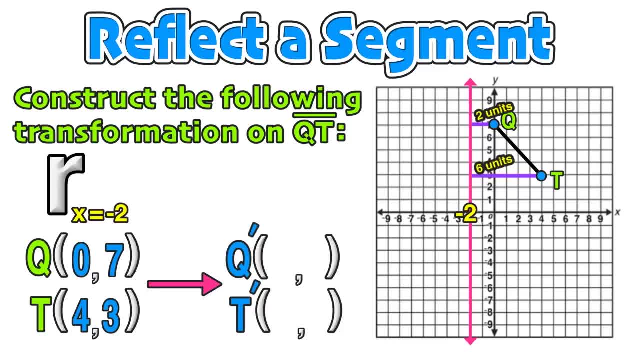 We see that the point q is two units away from the line of symmetry, x equals negative two and the point t is six units away. We can go ahead and repeat those distances on the other side of the line of symmetry and plot the new points of q' and t'. 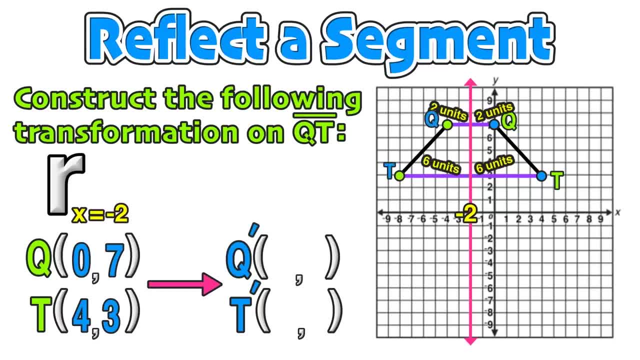 Now we can construct the image of the reflection. We can now see that the point q is two units away from the line of symmetry x equals negative two. We can now see the line of symmetry x is a reflected line segment. We can now see the line of symmetry y is a reflected line segment. 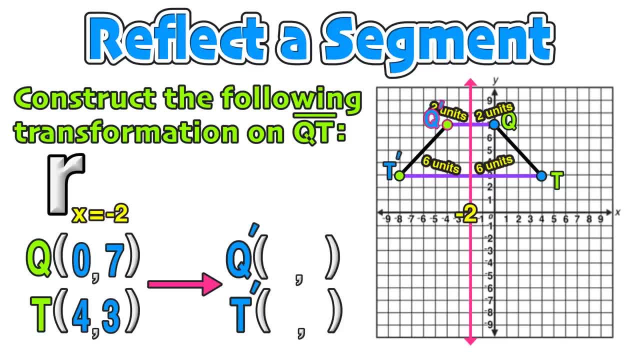 Q' has coordinates of negative four, seven, and t' has coordinates of negative eight, three. Now we can go ahead and try to reflect line segment qt over the line of symmetry. y equals three, a horizontal line equation. Notice here that the point t is directly on the line of symmetry. 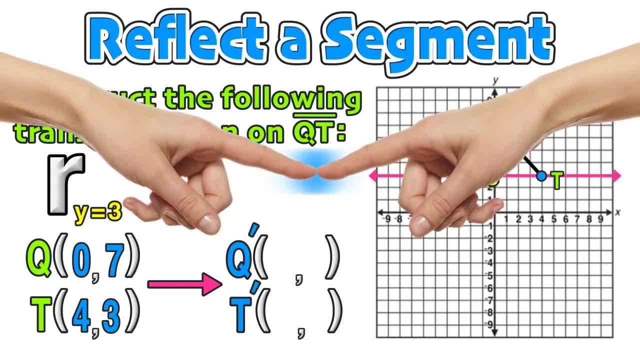 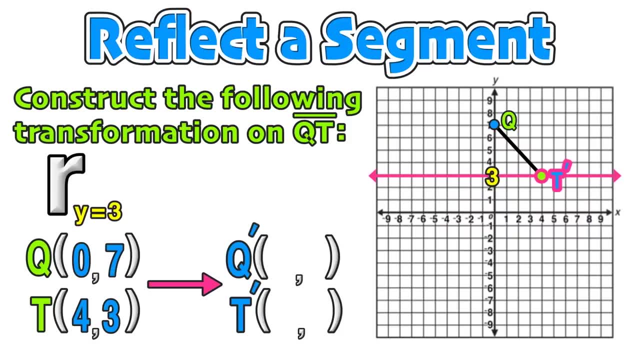 Just like pressing your finger up to the surface of a mirror and having it appear that another hand is directly touching it. having a point directly on the line of symmetry will have it stay on the line of symmetry. So T' will have the same coordinates as T at 4, 3.. 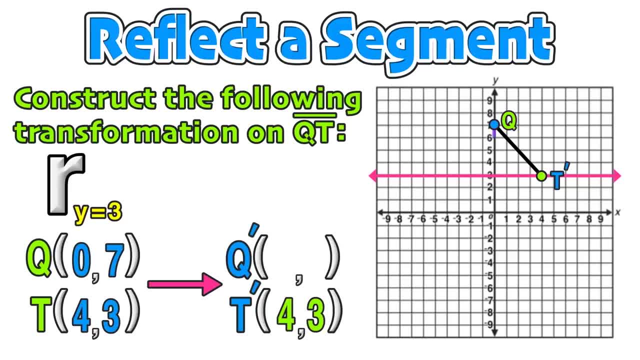 Now the other endpoint, Q, still needs to be reflected Again. we're just going to count how many units Q is from the line of symmetry. We count 4 units and we repeat that distance on the other side, again another 4 units and plot the image of Q'. 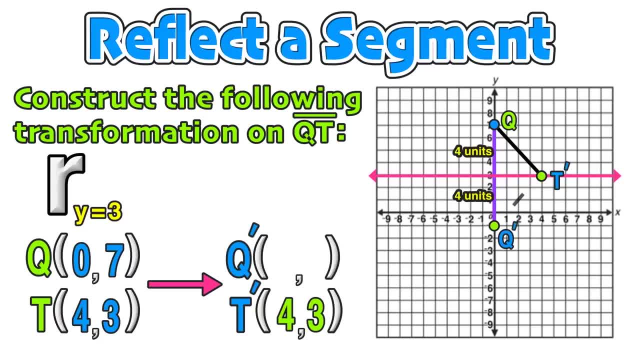 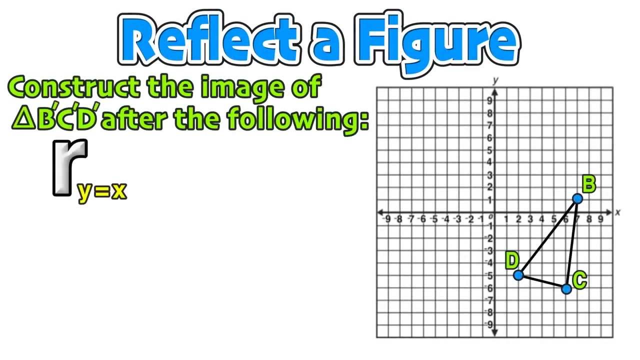 Finally, we can construct line segment Q' T' and identify the coordinates of Q' at 0, negative 1.. And finally, for our last example, we are going to count how many units Q is from the line of symmetry. And finally, we are going to take a shot at reflecting a figure. 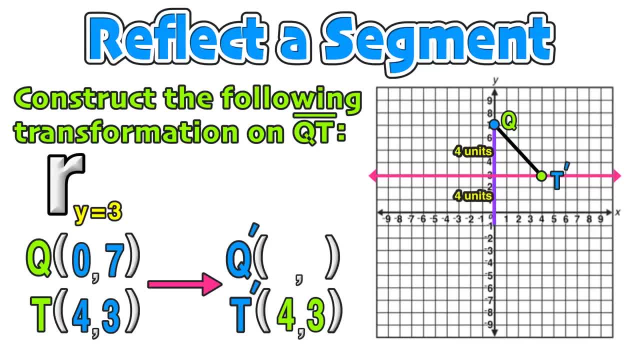 We count 4 units and we repeat that distance on the other side again another 4 units and plot the image of q'. Finally we can construct line segment q' t' and identify the coordinates of q' at 0, negative 1.. 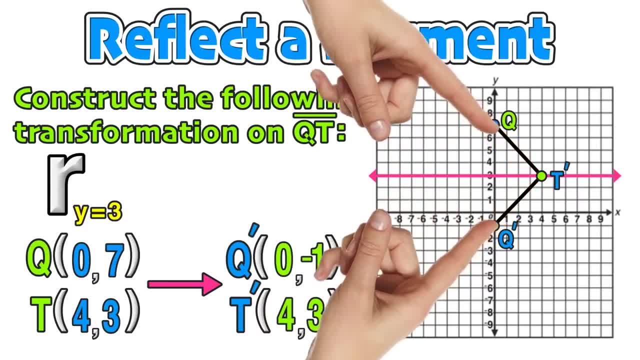 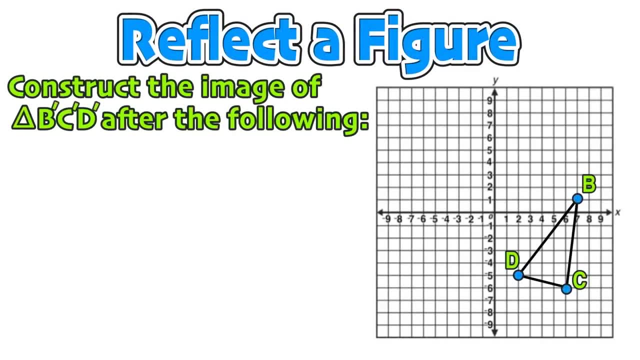 Now we can go ahead and repeat those distances on the other side- again another 4 units- and plot the image of q'. Finally, we can construct line segment q' t' and identify the coordinates of q' at 0, negative 1.. And finally, for our last example, we are going to take a shot at reflecting a figure. 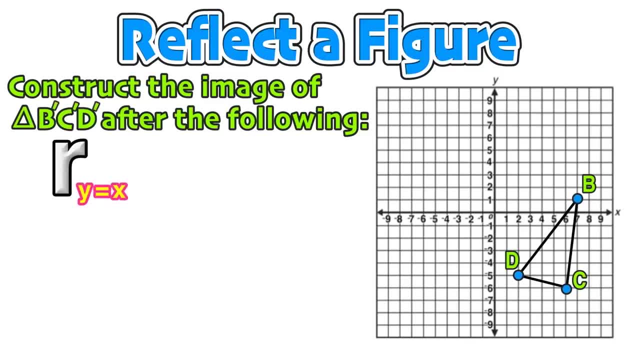 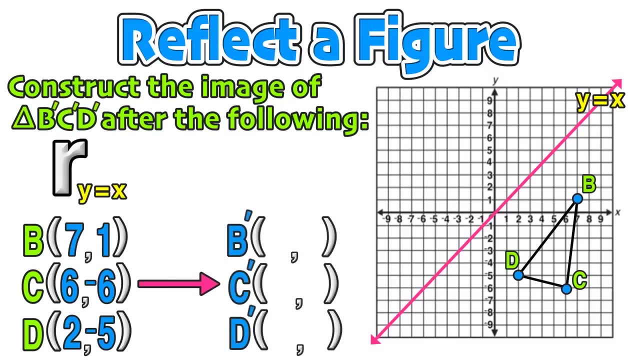 In this case we will be reflecting Triangle BCD. across the line Y equals x. We can start by writing down the coordinates of the vertices of Triangle BCD. We could start by counting on our alright. We've multiplied three times against. Now we're counting thrice on our answer. 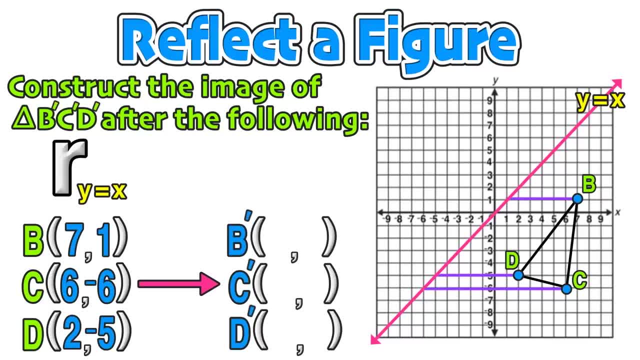 6 times y minus 2 equals 10 over 10 times y times 2.. a horizontal path: how many units each point is away from the line of symmetry? We see that b is 6 units away, d is 7 units away and c is 12 units away. 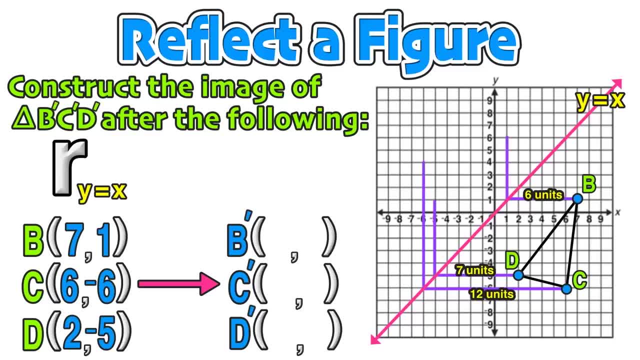 Now, since y equals x is a vertical line equation, when we count on the other side of the line of symmetry, we are going to move vertically. So we started horizontally on one side and now we are going to count vertically on the other side. By matching the same number of units for each corresponding point, we can find the coordinates. 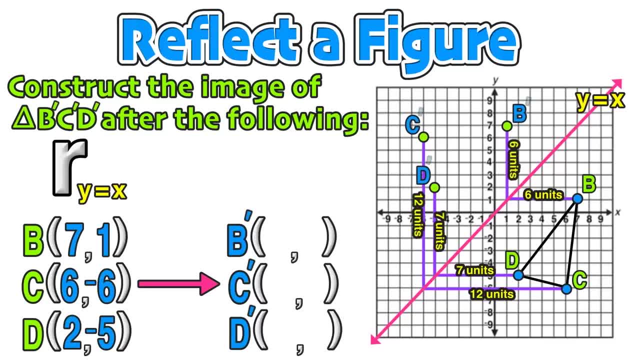 of b', c' and d'. Finally, we can construct the reflected figure: the coordinates of b' at, the coordinates of c' at and the coordinates of d' at. Now we can compare the preimage and the image after the reflection by turning the graph. 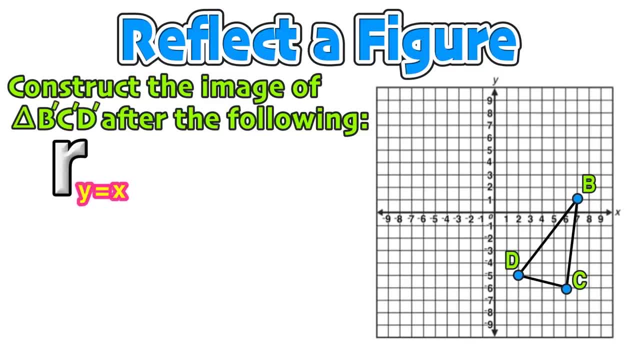 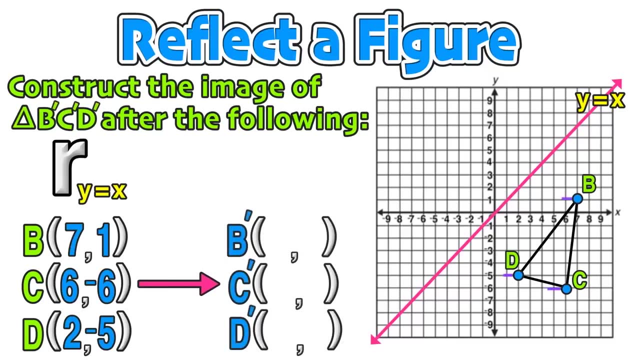 In this case we will be reflecting triangle BCD across the line Y equals X. We can start by writing down the coordinates of the vertices of triangle BCD. We can start by counting on a horizontal path: how many units each point is away from the line of symmetry? 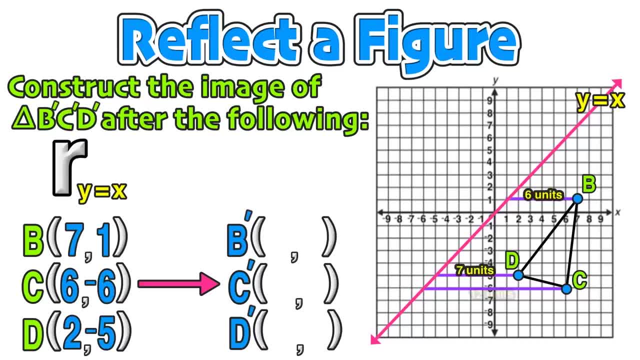 We see that Q' T' is 0, negative 1.. We can also see that B is 6 units away, D is 7 units away and C is 12 units away. Now, since Y equals X is a vertical line equation, when we count on the other side of the line of symmetry, we are going to move vertically. 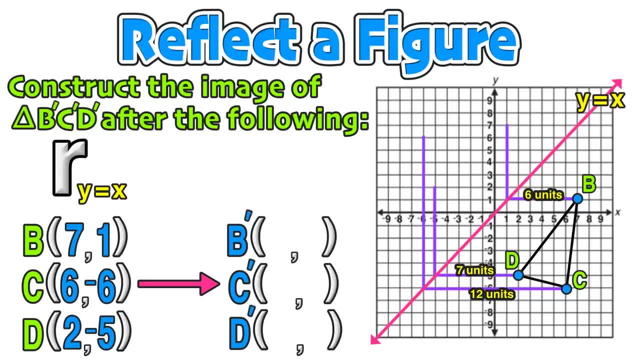 So we started horizontally on one side and now we are going to count vertically on the other side. By matching the same number of units for each corresponding point, we can find the coordinates of B', C' and D' Finally, we can construct the reflected figure: the coordinates of B' at 1, 7,, the coordinates of C' at negative 6, positive 6, and the coordinates of D' at negative 5, 2.. 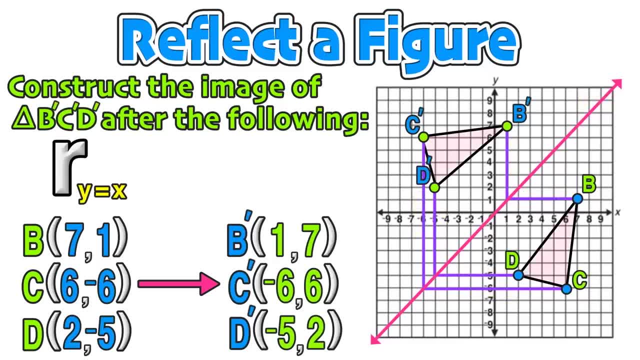 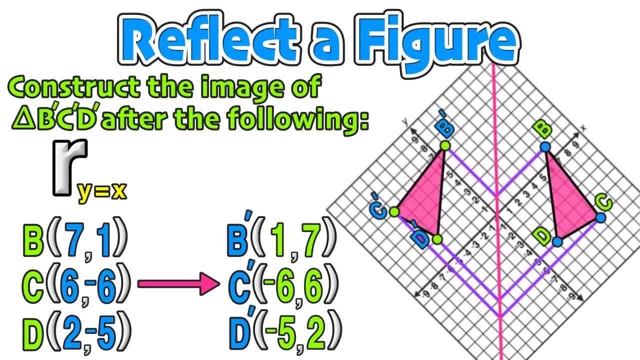 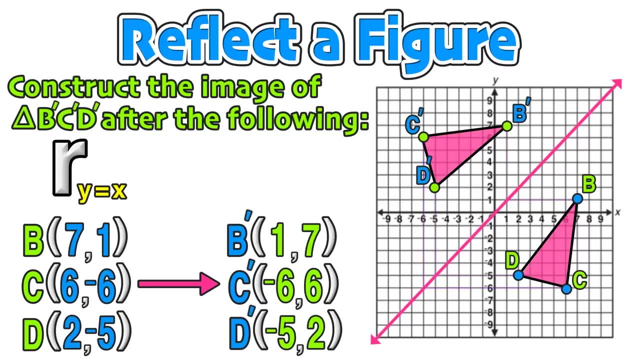 Now we can compare the preimage and the image after the reflection by turning the graph and seeing just how these two figures are reflected over the line. Y equals X. Notice the coordinates of B at 7, 1, and B' at 1, 7,, C at 6, negative 6, and C' at negative 6, 6, and D at 2, negative 5, and D' at negative 5, 2.. 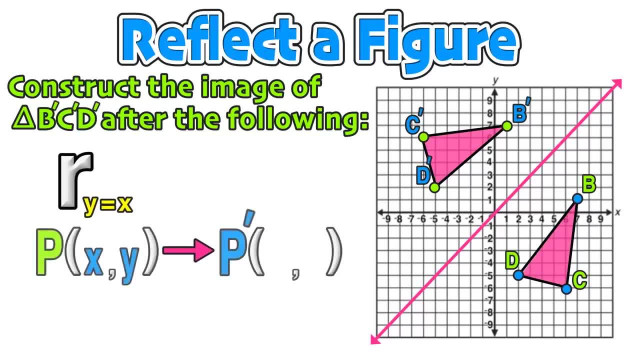 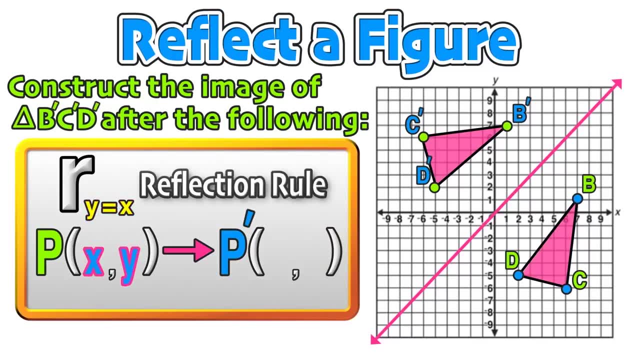 This relationship applies to any reflection over the line Y equals X. When you have a point P with coordinates, the X and Y coordinate values are switched. The Y coordinate value comes first and the X coordinate value comes second. The signs do not change. 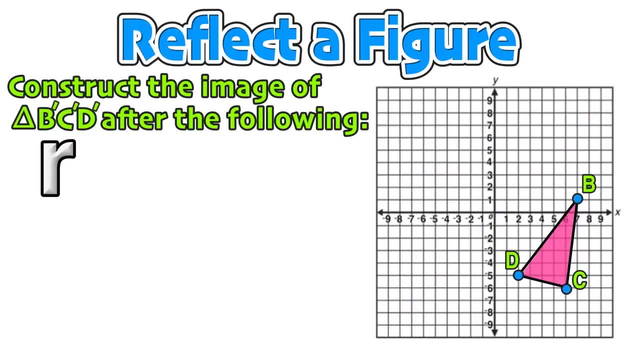 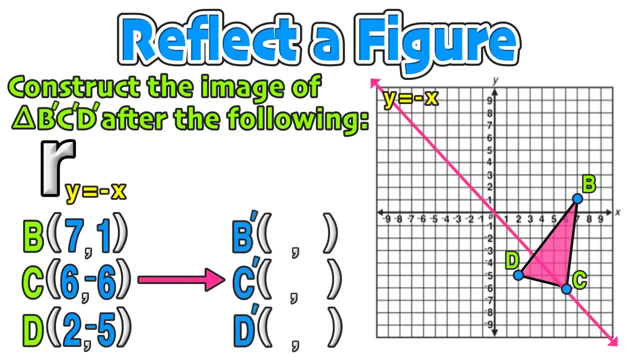 And now we can take a look at reflecting this figure over the line. Y equals negative X. Again, let's start by constructing the line of symmetry and writing down the coordinates of the vertices of triangle B, C, D. Notice here that the figure is resting on top of the line of symmetry. 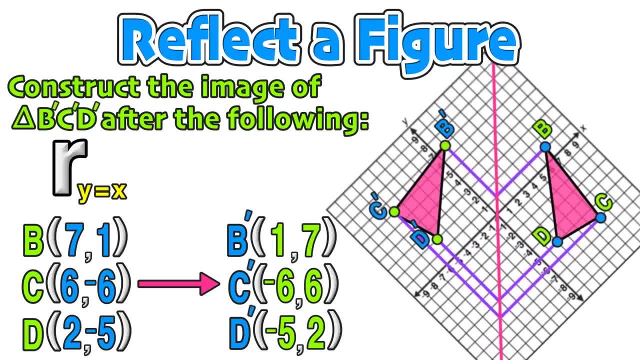 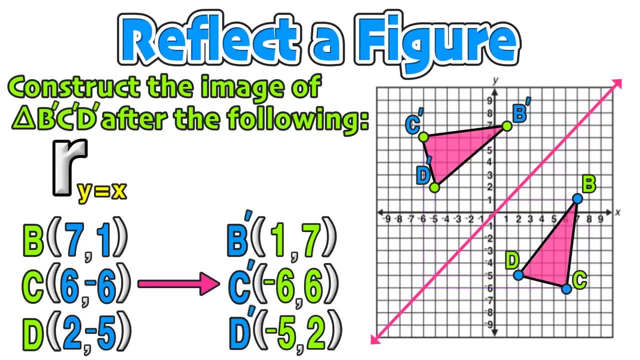 and seeing just how these two figures are reflected over the line y equals x. Notice the coordinates of b? at and b' at, c- at and c' at, and d' at and d' at. This relationship applies to any reflection over the line y equals x. 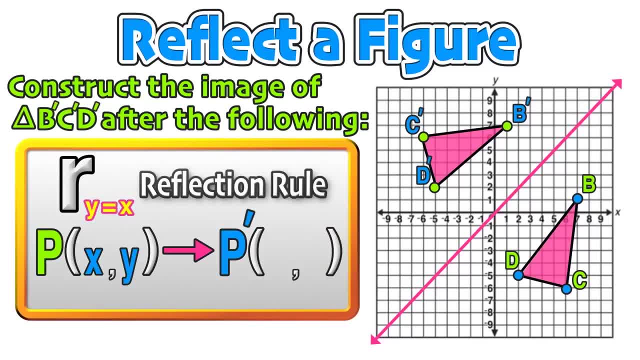 Now we can see that b' at, c' at, d' at and d' at. When you have a point p with coordinates xy, the x and y coordinate values are switched. The y coordinate value comes first and the x coordinate value comes second. 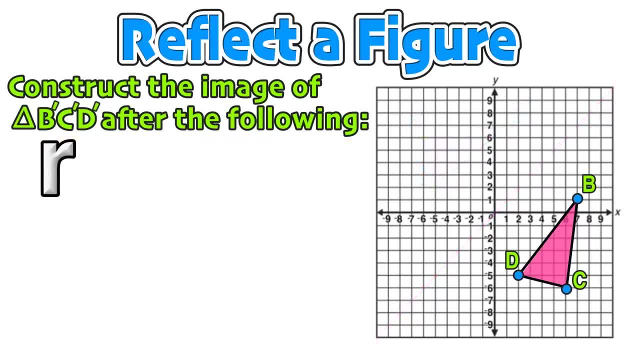 The signs do not change, And now we can take a look at reflecting this figure over the line. y equals negative x. Again. let's start by constructing the line of symmetry and writing down the coordinates of the vertices of triangle b, c and d. 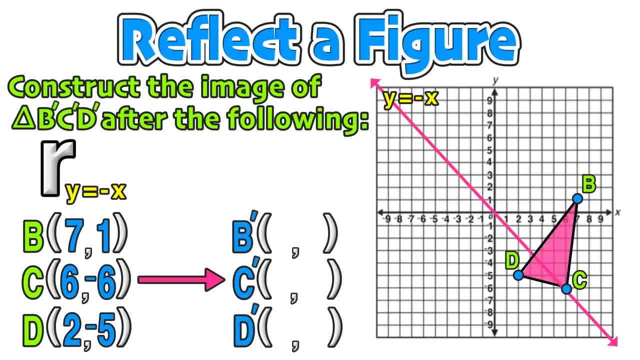 We can see that the lines are not the same. We can see that the lines are not the same. Notice here that the figure is resting on top of the line of symmetry and is in two different regions. Now we know that since point c is directly on the line of symmetry, c' will have the 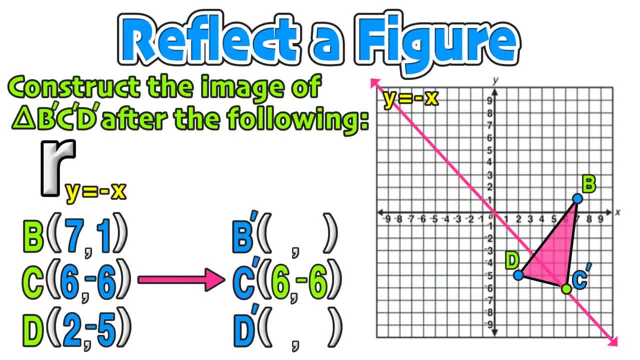 same coordinates of Next. point b is located above the line of symmetry. We'll start by counting the number of units horizontally. it is, away from the line of symmetry, 8 units. Next step is to repeat that same number of units vertically, on the other side of the. 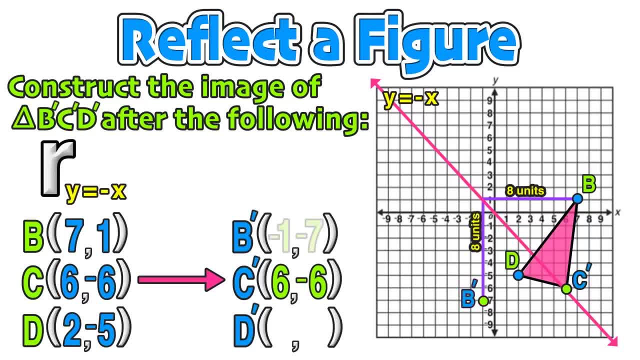 line of symmetry to find the coordinates of b'. And finally, since point d is below the line of symmetry, we'll start by counting how many units vertically it is away from the line y equals negative x, And then repeat that distance moving horizontally above the line of symmetry. 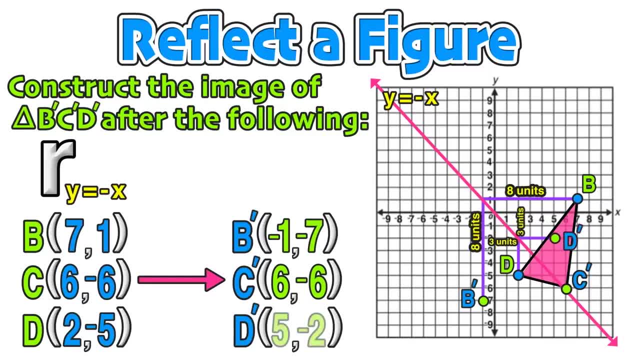 Now we have the coordinates of d'. at Next step is to repeat that same number of units vertically on the other side of the line of symmetry to find the coordinates of b' By connecting those vertices we construct the image of b', c', d' to create a very 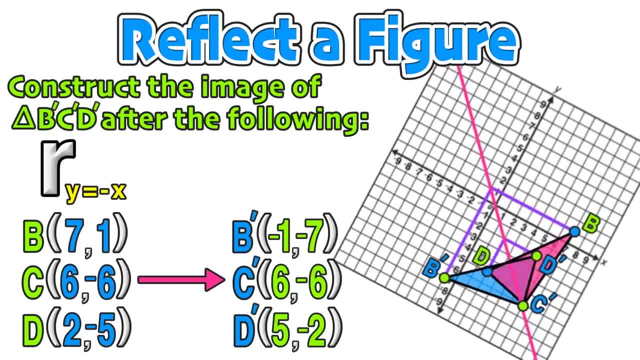 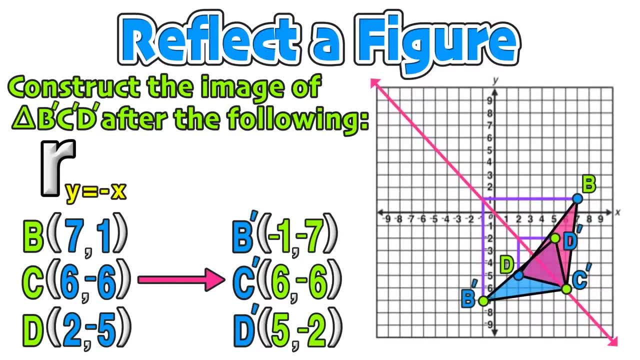 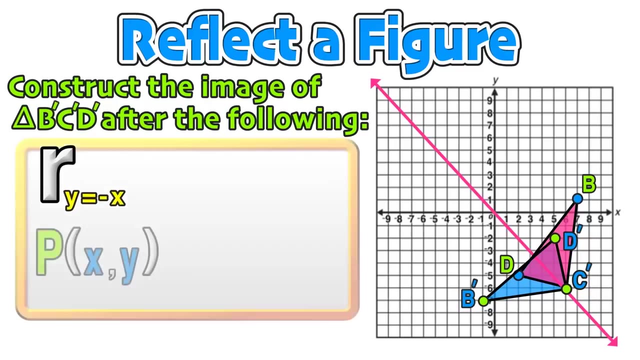 interesting picture. We can rotate the graph to better visualize what this reflection looks like. Now we can compare the point b with coordinates and b' at c remained unchanged, and d with coordinates. If you notice, for this relationship when reflecting any point over the line y equals. 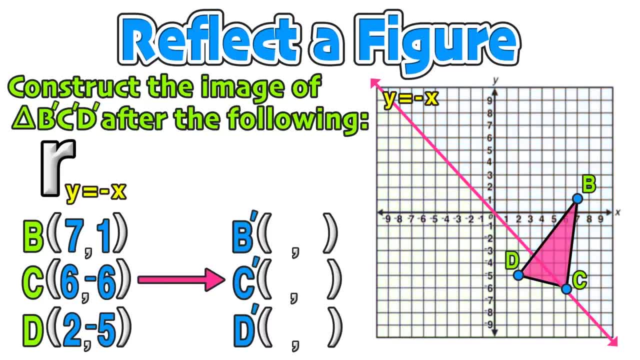 And is in two different regions. Now we know that, since point C is directly on the line of symmetry, C' will have the same coordinates of 6, negative 6.. Next, point B is located above the line of symmetry. We'll start by counting the number of units horizontally. it is away from the line of symmetry, 8 units. 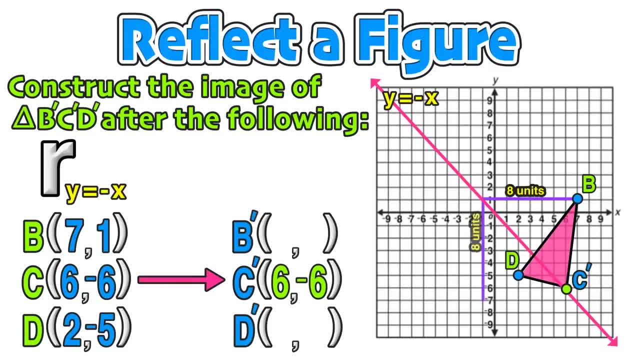 The next step is to repeat that same number of units vertically on the other side of the line of symmetry To find the coordinates of B' And finally, since point D is below the line of symmetry, we'll start by counting how many units vertically it is away from the line. Y equals negative X. 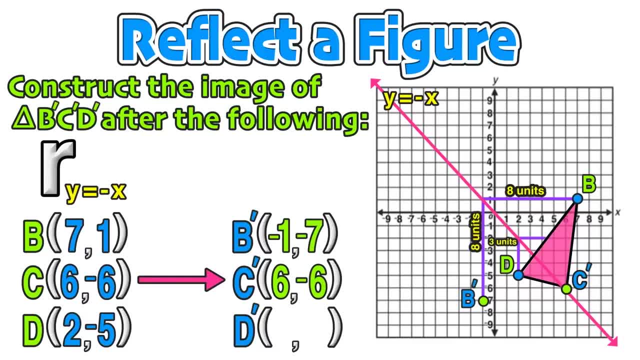 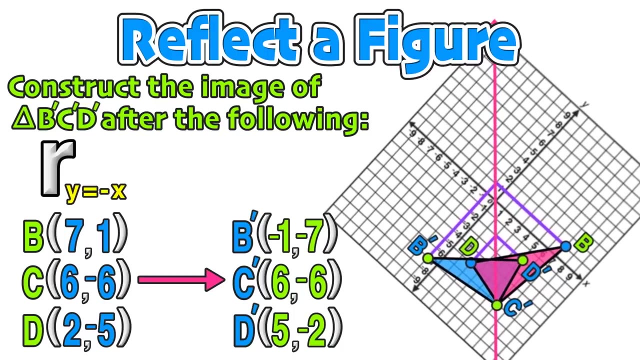 And then repeat that distance moving horizontally above the line of symmetry. Now we have the coordinates of D' at. By connecting those vertices we construct the image of B', C', D' to create a very interesting picture. We can rotate the graph to better visualize what this reflection looks like. 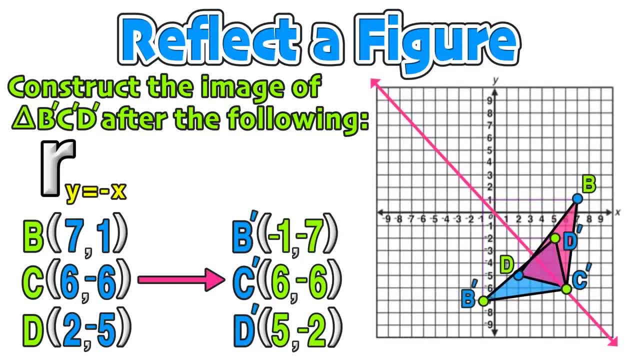 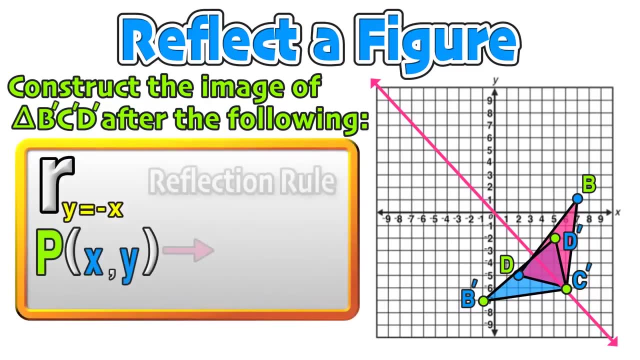 Now we can compare the point B with coordinates and B' at C remained unchanged and D with coordinates to D' If you notice, for this relationship, when reflecting any point over the line Y equals negative X, the X and Y values are switched and negated. 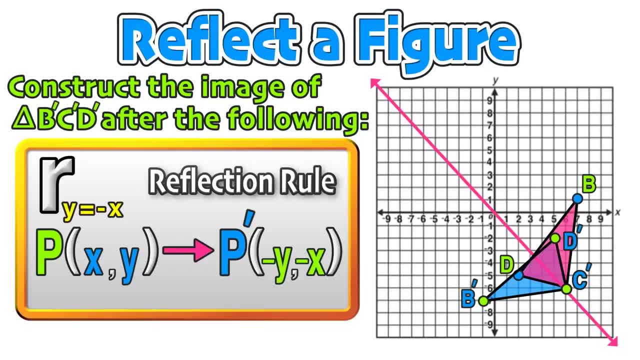 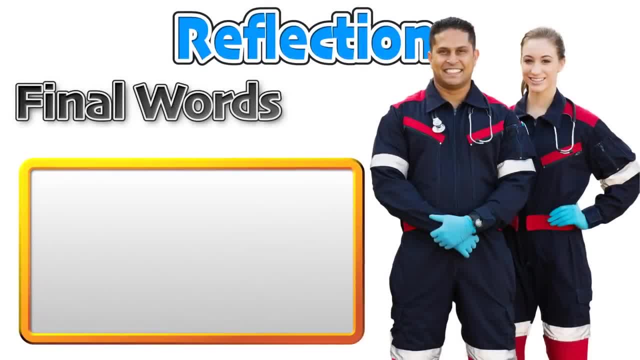 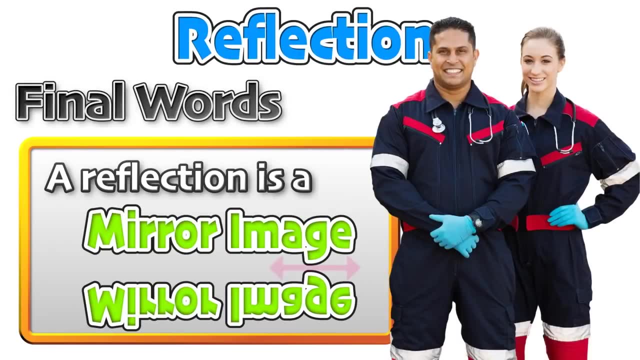 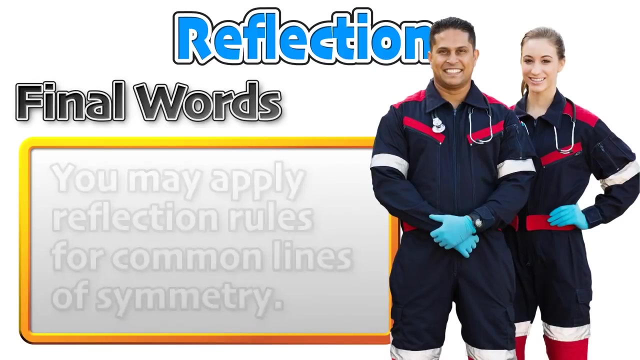 So XY becomes negative, Y negative, X. And now our final words on reflections. A reflection is a mirror image across a specified line of symmetry. For these transformations you may apply reflection rules for common lines of symmetry. These common lines of symmetry include the X and Y axis. 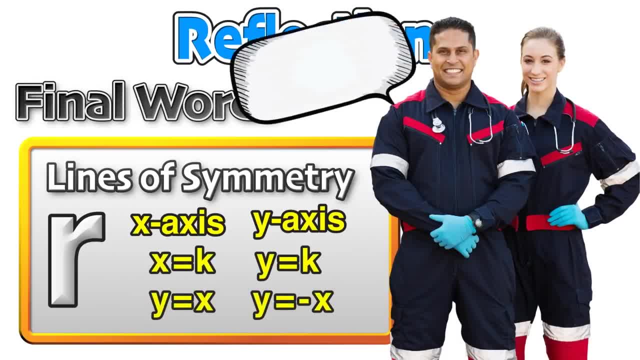 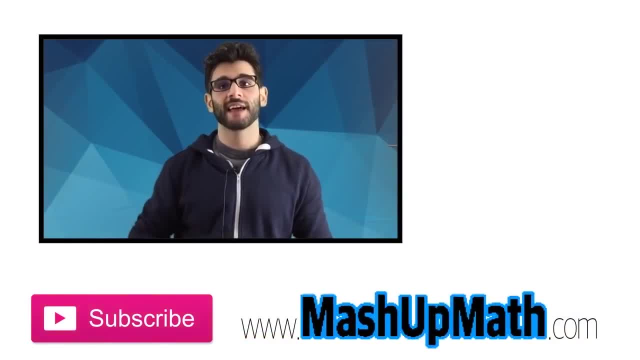 the lines X equals K and Y equals K and the line Y equals X and Y equals negative X. Thanks a lot, guys, for checking out that lesson. Please subscribe to our YouTube channel and head on over to mashupmathcom for more content and practice activities.